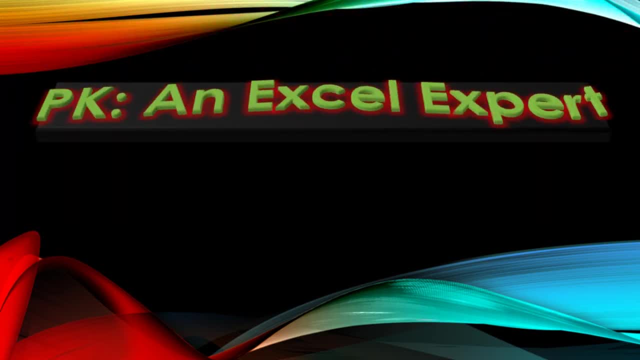 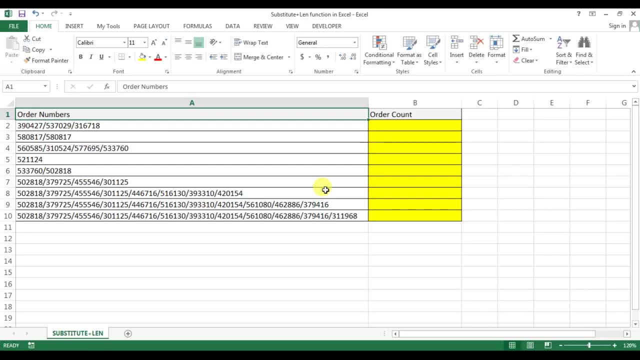 Hello friends, welcome back. My name is Priyantra Kumar and today we will learn how to use substitute function in Microsoft Excel. Friends. yesterday one of my friend asked me a question regarding this data. So these are the order number, and these order numbers are separated by the forward slash. 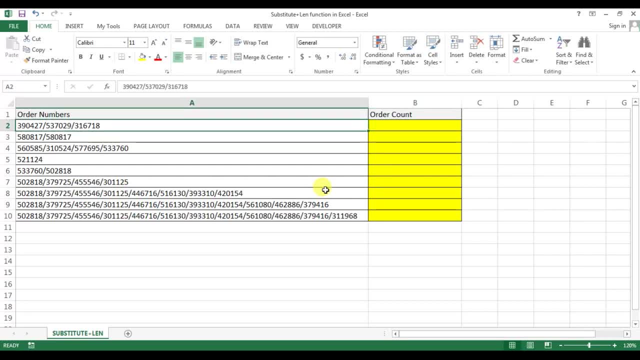 So if we have to count the how many orders are available in a cell, then how we can use it by formula. So, friends, I have told him about the substitute function we can use here, So I thought I should share it with you. So that's why I'm creating this video. So, friends, here we will use. 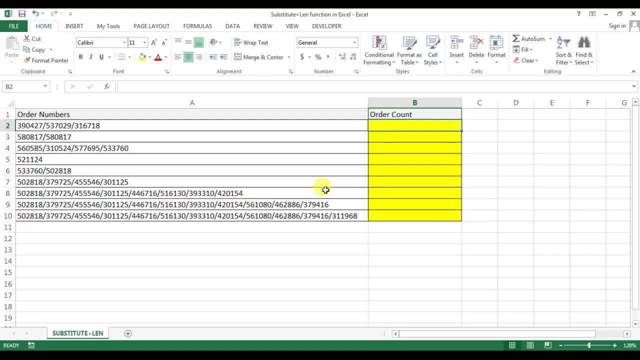 a substitute function, So I'll tell you in detail. So, first of all, what we will do, we'll get the length of this text. So the length of this text is 20 characters. right Now we will use substitute Substitute, then this text and the old text will take these less, which is used as a separator here. 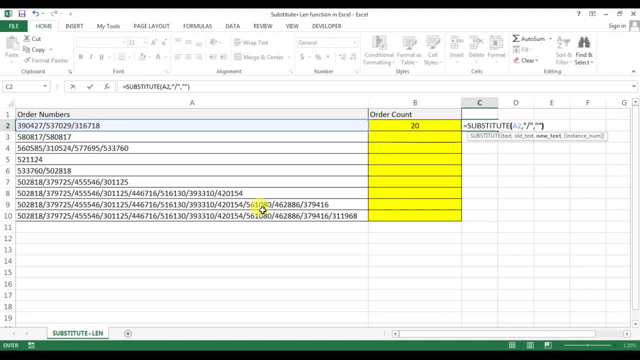 Then the new text will be blank. So just close the bracket Now it will give the same text, but it will replace the slash with the blank only. So now we will get the length of this. Now it is 18.. So because here is two slash which has been replaced with the blank. that's why 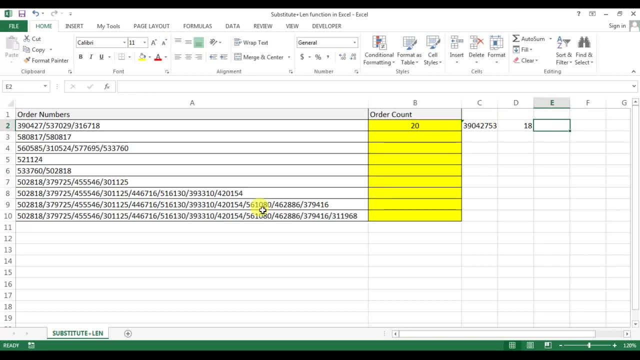 the length is now 18.. Okay, now I can get the number of slash, how many cell SSR in the data. So that is two. Now we can check. if number of lessons is two, then my order number will be three. The order number is two, but the last is one. Okay, so what I will do? I have used plus one.